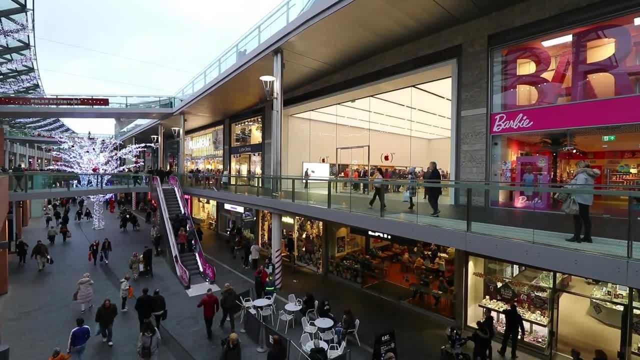 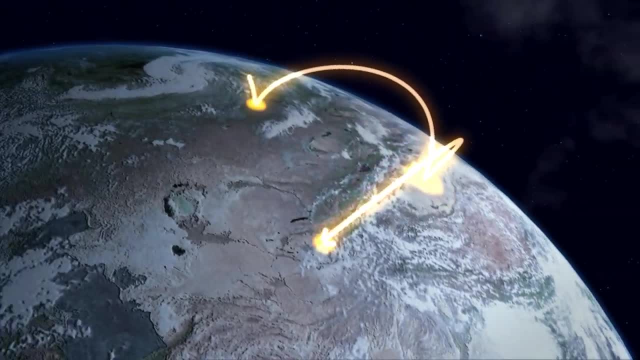 goods and services and specific skills, But at the same time, they also lack certain resources and skills as well. This leads to countries to trade with other countries around the world, And when countries trade, it allows them to become more specialized and it increases the 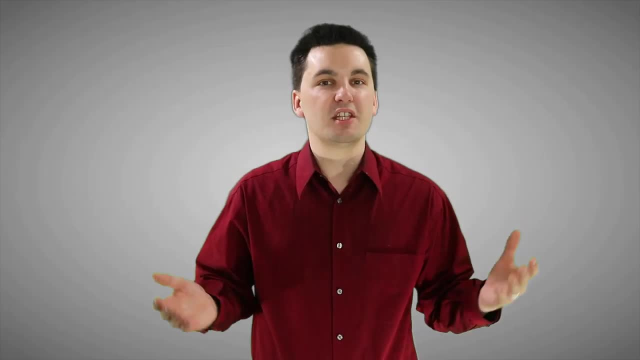 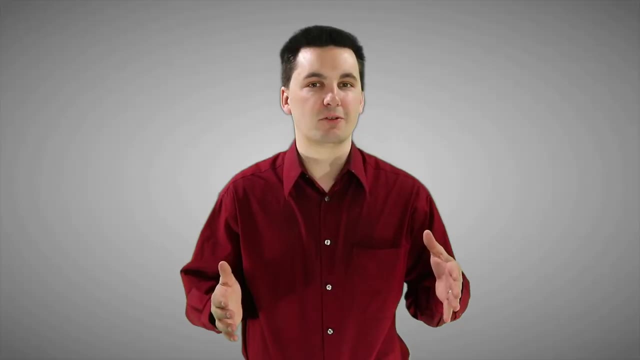 amount of goods and services for the country's citizens. Plus, we can see that both countries that participated in the trade gain more economic and also social opportunities for their citizens. When looking at trade, we can see that countries that have a stronger trade relationship with other countries have a stronger trade relationship with other countries. 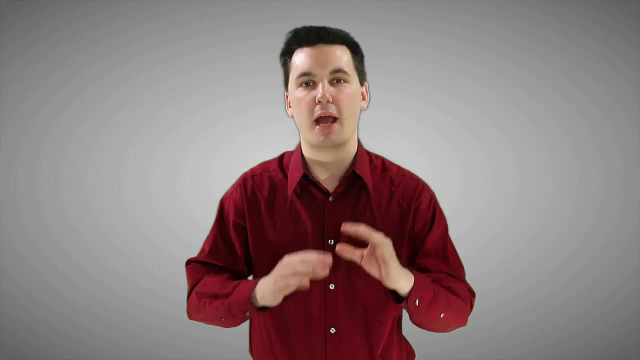 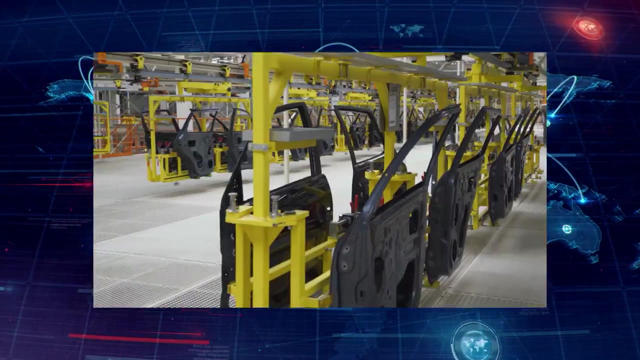 Trade Complementarity Index score will often see more interaction between each other. Trade Complementarity is a trade index that looks at the interaction between two countries that provide goods and services or resources to meet the needs, wants and demands of another country. We can see: 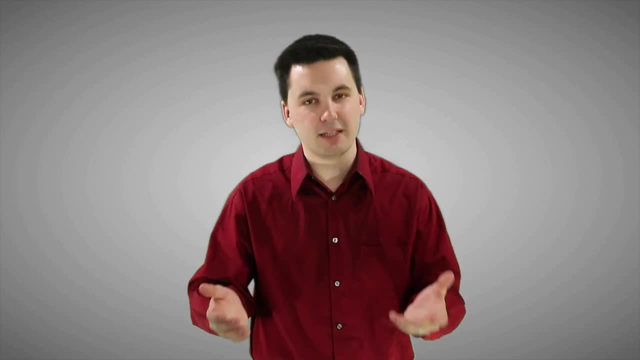 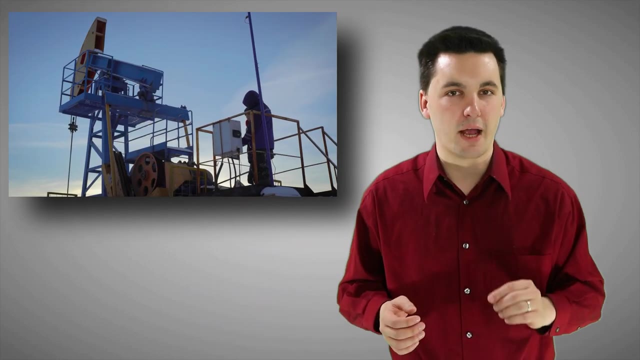 this, for example, when looking at the United States and oil. The United States needs a lot of oil to support the American economy and the United States imports oil from around the world. Canada is the largest foreign supplier of crude oil to the United States. We can see that the 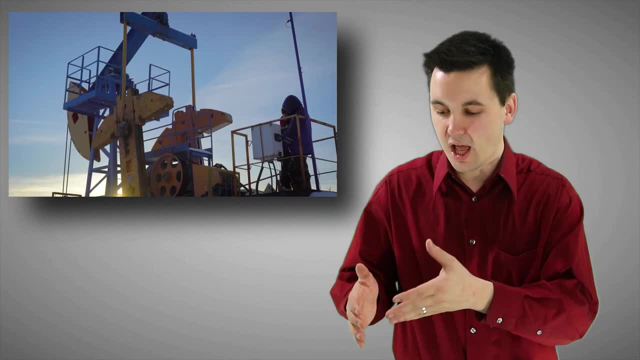 United States is the largest foreign supplier of crude oil to the United States. We can see that the United States has a need for crude oil and Canada has a supply to fill that need. Another reason why countries trade is because of comparative advantage. Every country business. 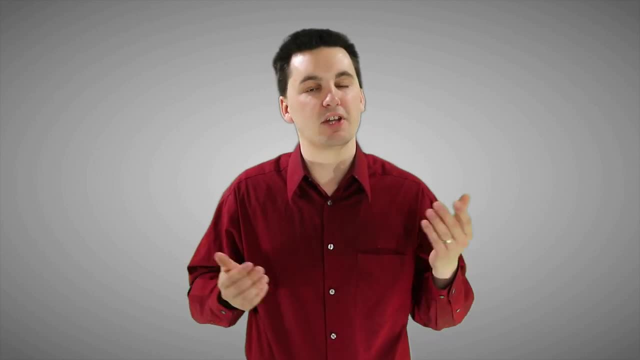 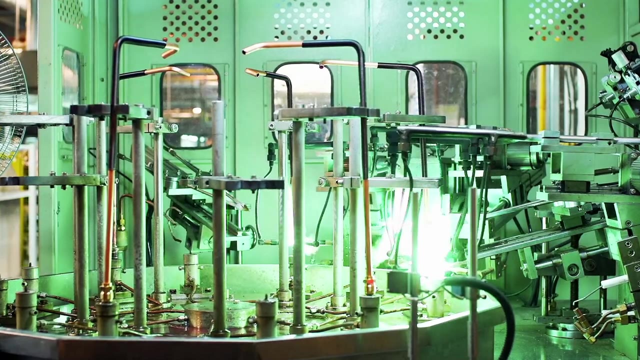 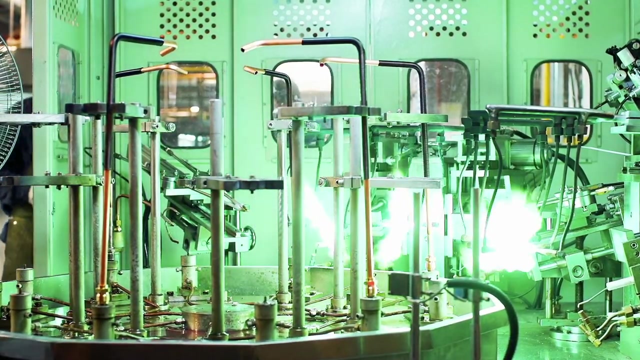 and person is better at certain tasks compared to other people. When countries are more efficient at producing a product over another country, they have a comparative advantage. Countries that have a comparative advantage in the production of a certain good should produce that good and trade with other countries. This allows them to maximize their efficiency. When countries trade, 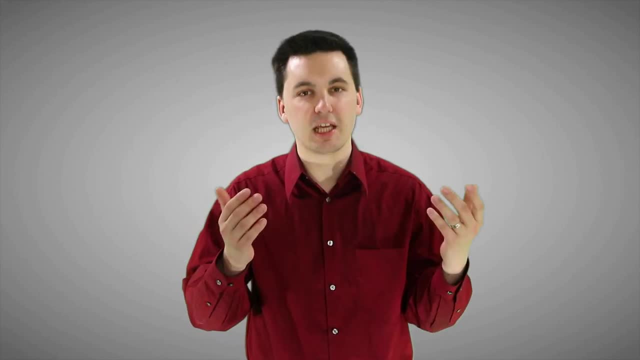 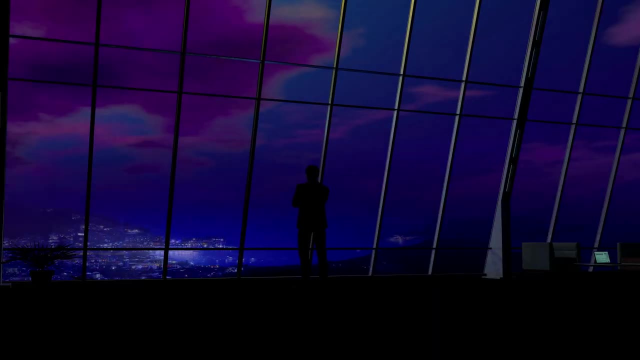 with other countries. it allows them to specialize more and it allows them to gain more access to different goods and services. This can increase the standard of living in a country and lead to economic prosperity. We can see that countries today are involved in complex trade networks that 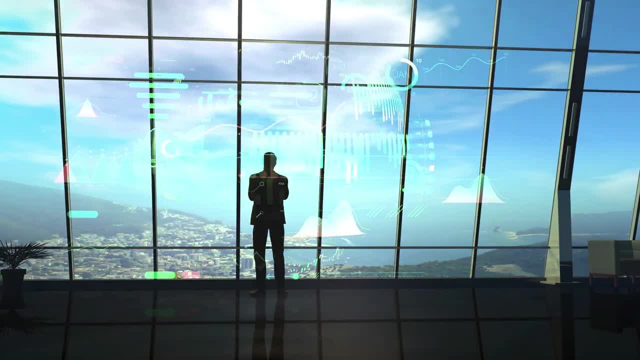 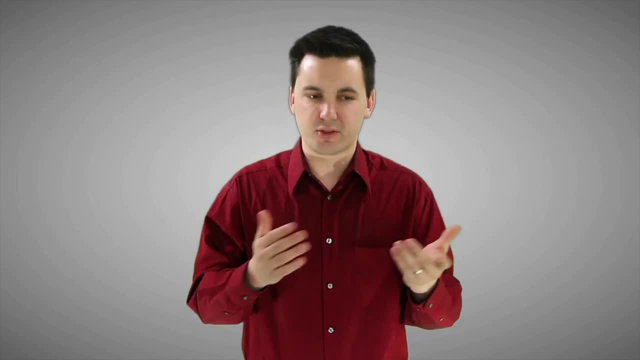 can lead to economic opportunities but, at the same time, can also lead to trade disputes. For example, you might have heard how the United States and China have a trade deficit and how the United States and China have been using tariffs to try and balance the scale. But what does this? 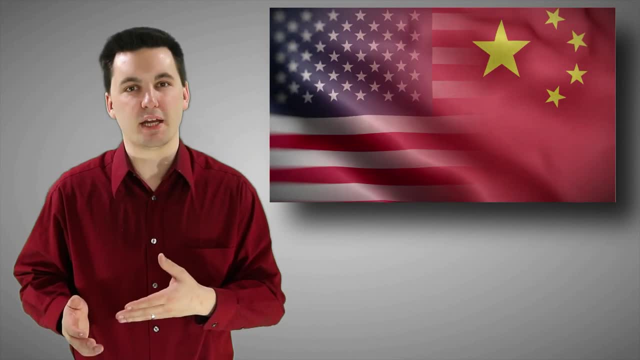 actually mean. Well, when you hear that the United States and China have a trade deficit, you know that the United States has a trade deficit with China. What that means is the United States purchases more goods from China than China purchases from the United States. Many economists argue that trade deficits aren't the end of the world, since we participate in these trade deals voluntarily. If the United States didn't value the goods from China more than our own money, then we wouldn't have traded with China in the first place. Now I also mentioned tariffs earlier. Tariffs are often used to try and motivate companies to 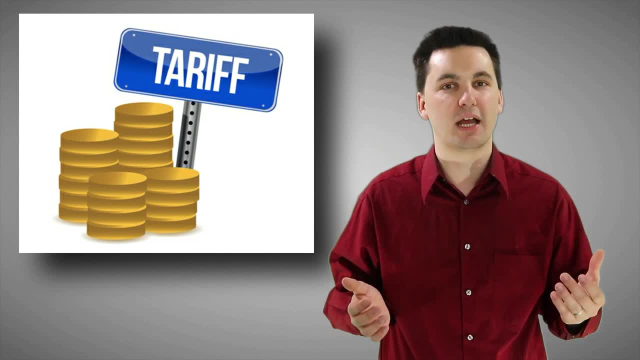 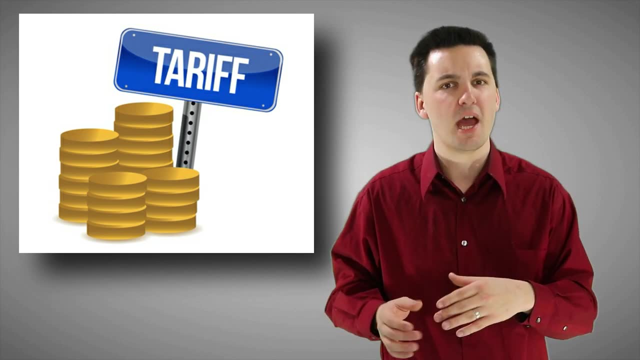 move back to domestic production. It tries to incentivize companies to make products within the country that's implementing the tariff. A tariff is a tax that gets put on imports. Imports are goods that are being shipped into a country. That tax makes it more expensive to. 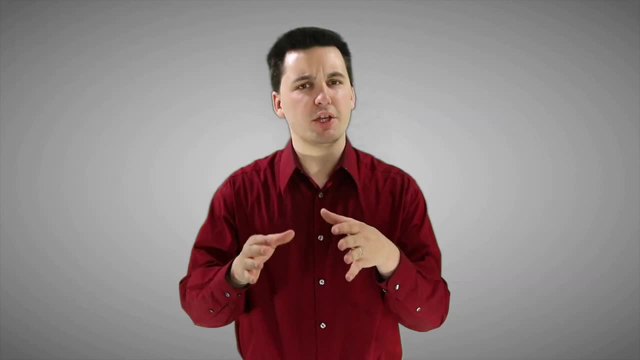 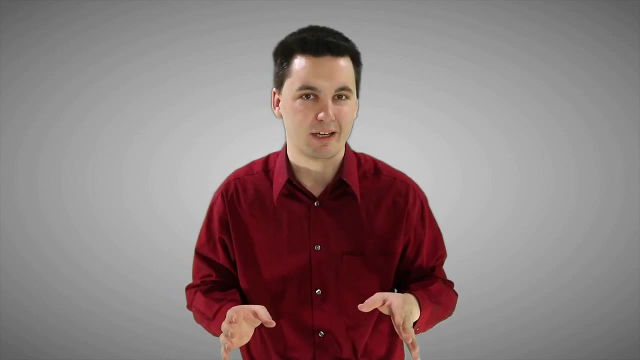 produce those products outside the country's boundaries. Now, one thing with tariffs I do want to clarify is the tariff that's being put in place isn't being paid by the country itself. No, the government isn't paying it, It's actually the consumers or the businesses Oftentimes. this makes the production more expensive, So companies have to raise the prices of their products. This then makes it so when you go to the store and you're buying a product that was imported, it normally costs more, since companies will pass on that cost that they had to pay for importing. 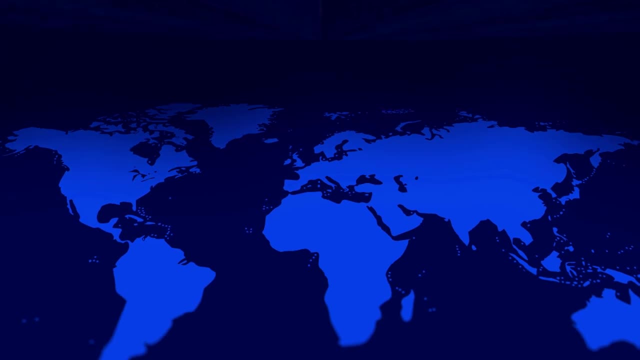 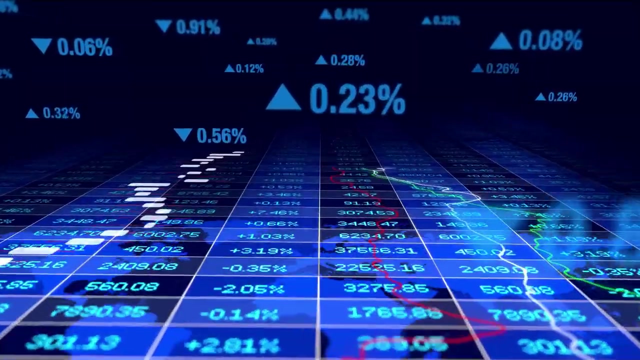 the products onto the consumer. Now, today, when we're looking at economies around the world, we can see that the majority of economies have some degree of a free market. Each country around the world is different and some economies are more open than others. However, generally, 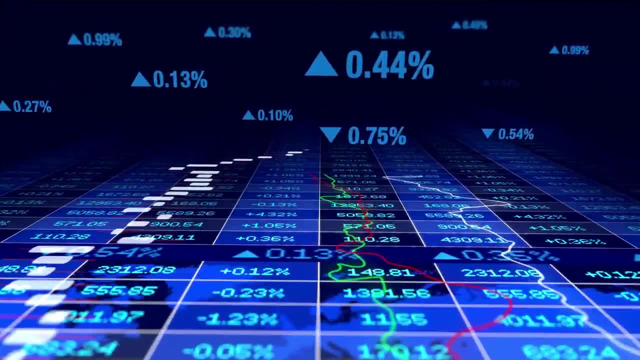 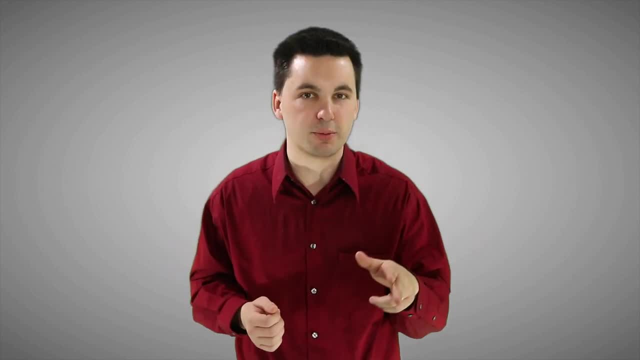 we can see that countries favor free market economies more than command economies. Command economies are economies that are controlled by the state, which means that they are controlled by the state- The decisions of what to produce, for whom to produce and where to produce. 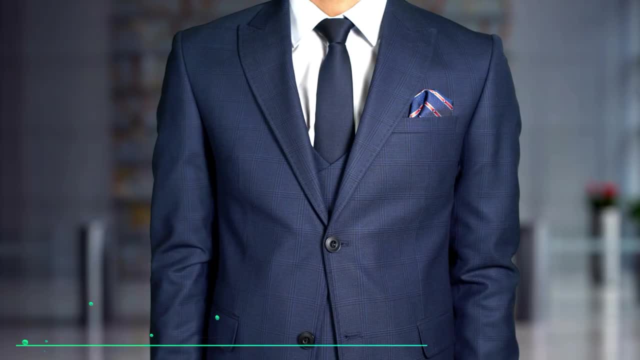 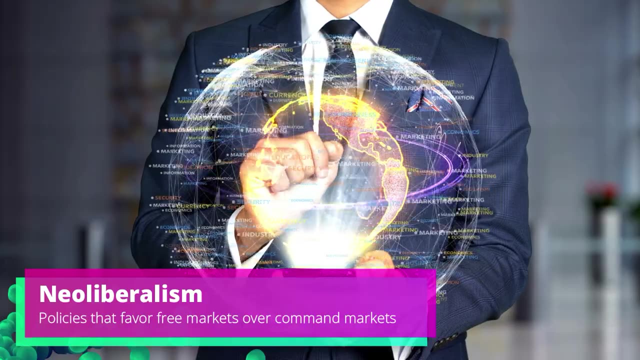 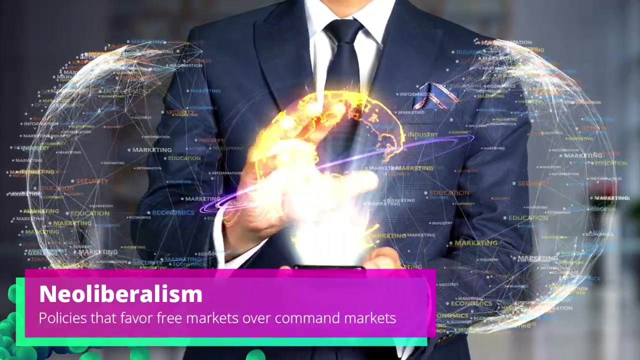 are all decided by a government, not by the free market. Today, when looking at free markets around the world, we can see that neoliberalism is becoming more and more popular. Neoliberal policies work to try and make trade between different countries easier. They reduce taxes and tariffs and try to promote trade between countries. 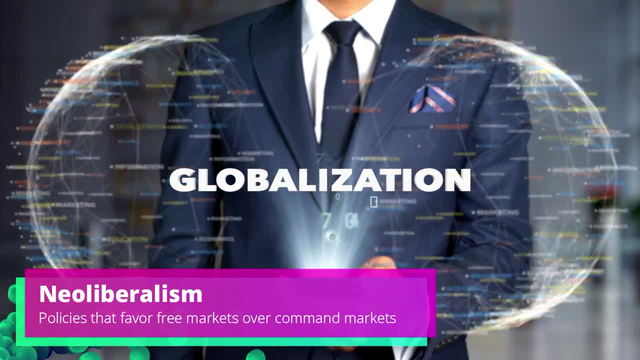 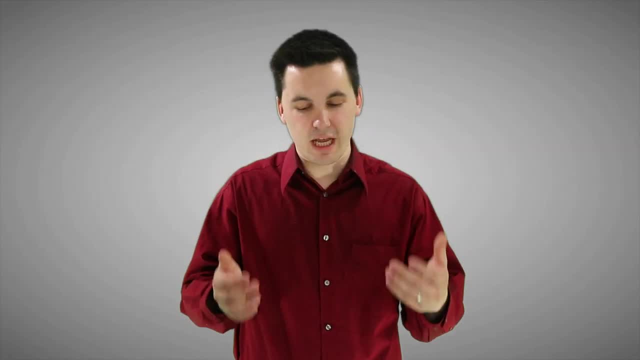 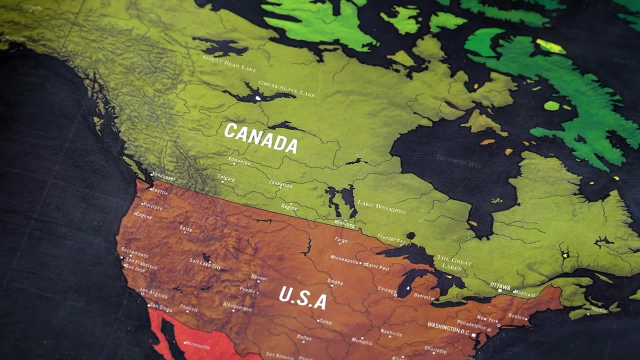 These policies favor free market economies, with privatization over business instead of government controlled economies. We can see that supernational organizations around the world have been created with neoliberalism policies in mind: Agreements like NAFTA, now the USMCA, which seek to bring free 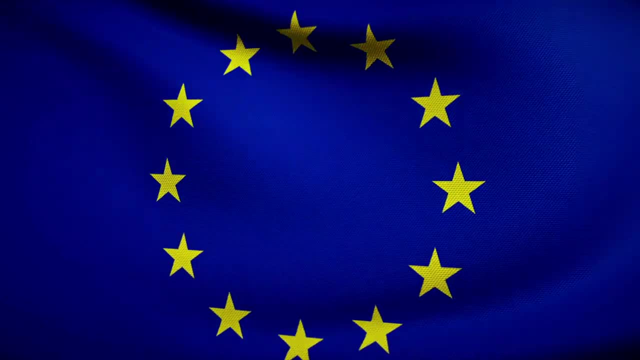 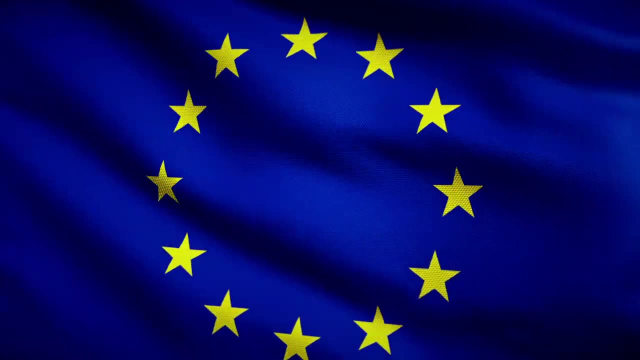 trade between Mexico, Canada and the United States, or the European Union, which created free trade between countries that are part of the union, all facilitate trade between different countries. We can look at the impact of the World Trade Organization, which seeks to promote. 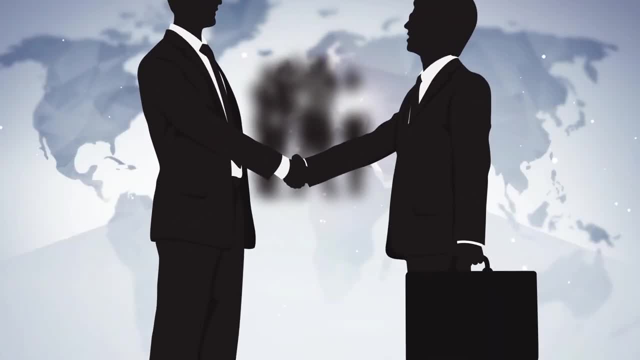 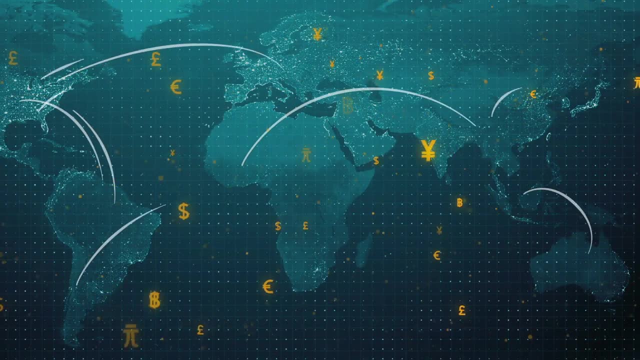 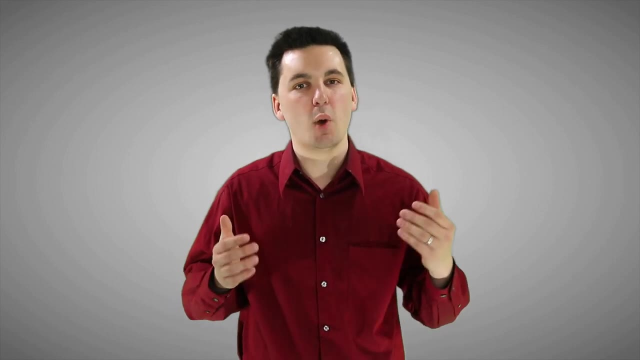 the international monetary fund, which seeks to create financial stability around the world and facilitate international trade and sustainable economic growth for countries all over the globe. This focus on international trade, globalization and supernational organizations has led to a higher standard of living for people all over the world. We've seen more goods and services become 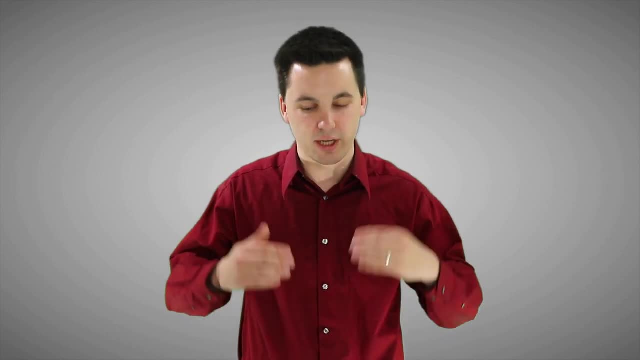 accessible to countries all over, along with new innovations that have driven more economic growth and prosperity. However, at the same time, this newly developed international monetary fund is a source of economic stability for the world. It has been a key part of the world's economic development and development. The world's economically connected 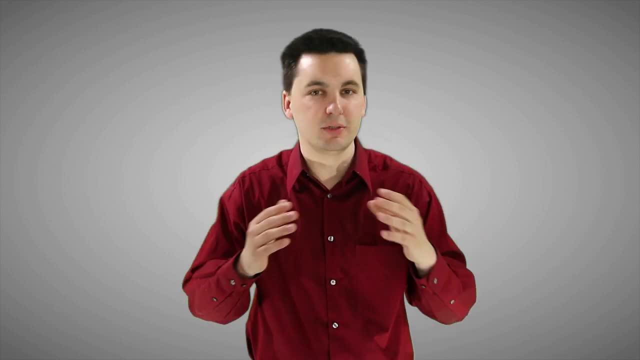 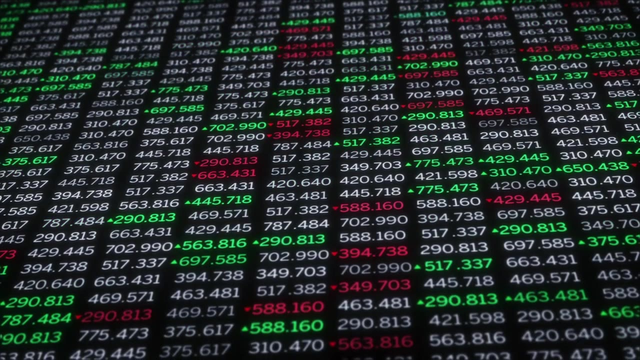 world also has some drawbacks. Economies today are supremely connected and what happens in one country now can have a ripple effect on the entire global community. For example, in 2008,, the world saw the global financial crisis, which diffused throughout the world. 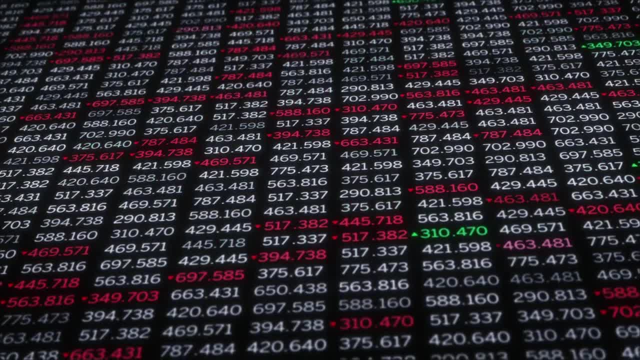 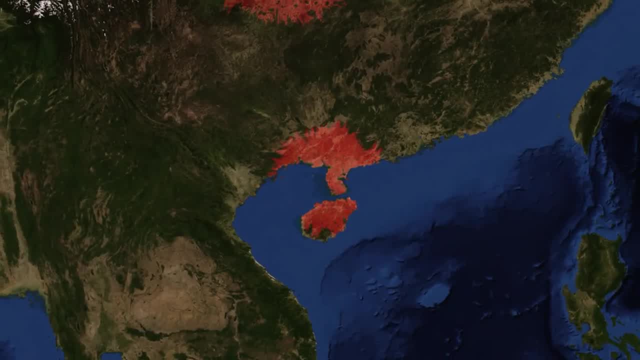 impacting almost every country's economy in the entire world. At the same time, we could also look at 2020, with COVID-19,, starting off originally in China, diffusing throughout the world. As the virus spread, economies shut down and we saw shortages. around the world because our newly connected world relied on these supply chains. Countries' productions now are directly connected and when the economy and production facilities in one country shuts down, it has a ripple effect on the rest of the global community. We could also look. at 2021, when the Suez Canal was blocked by a cargo ship. The blockage ended up costing global trade somewhere between the ballpark of six billion and ten billion dollars a week, Due to the Suez Canal being a significant choke point for global trade every single day over. 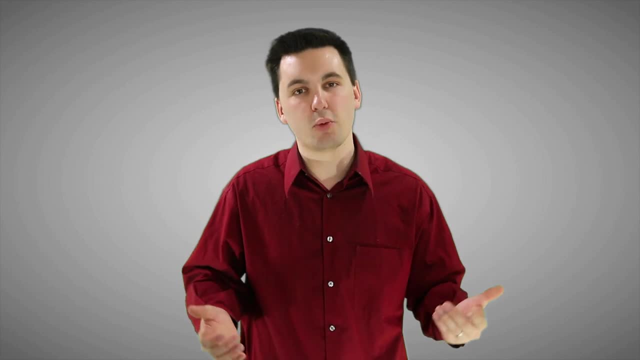 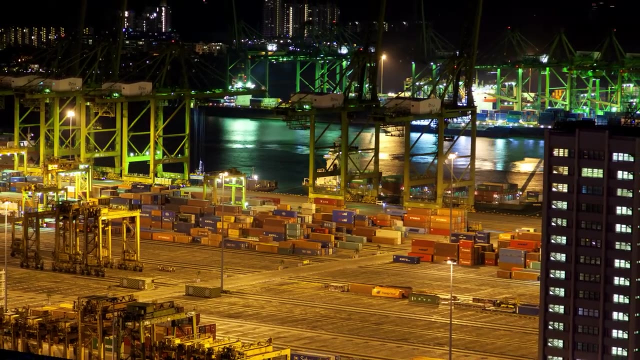 12 percent of global trade goes through the canal, And when that choke point was blocked, we saw major implications for the world economy. Today we can see that trade and the world economy impacts every level of society. On the local scale. we can see workers and small businesses. 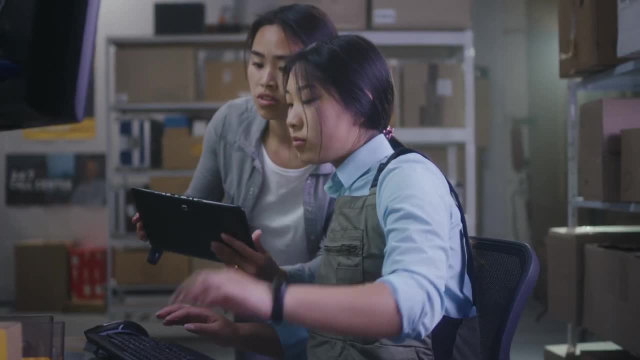 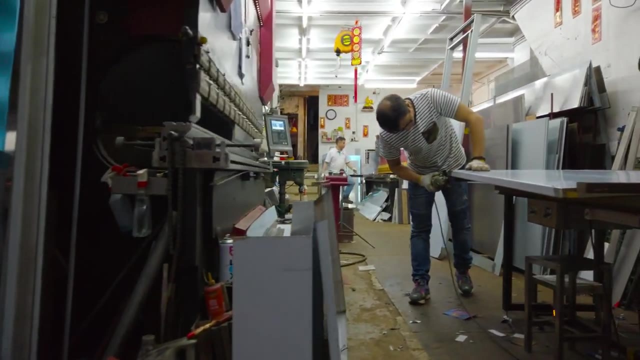 are no longer just competing for jobs and business within their own communities and their own towns. now they're competing with people across the globe, And this can lead to disparities between workers, as companies may favor countries that have cheaper labor And it might put a 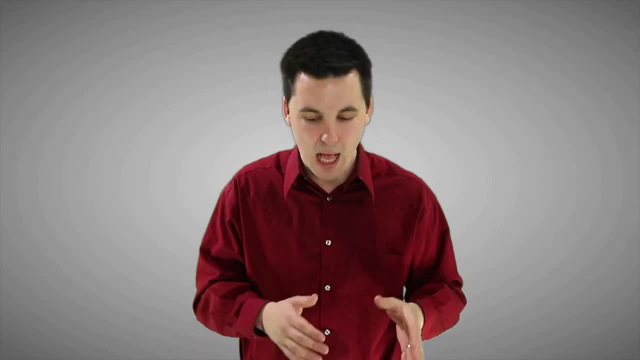 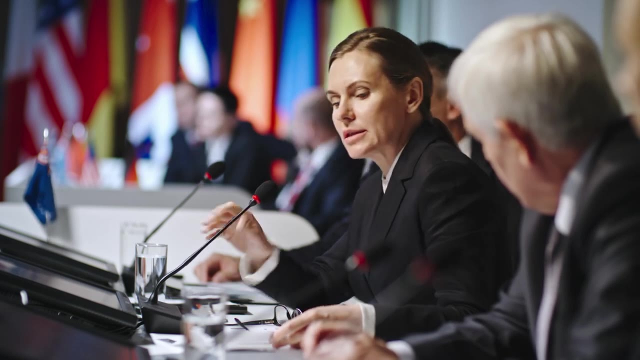 disadvantage on more developed countries as we see more offshoring of jobs as they start to go overseas. At the national scale, we can see how countries' entire economies now are connected to other countries around the world. What happens in one country will impact other countries, And this 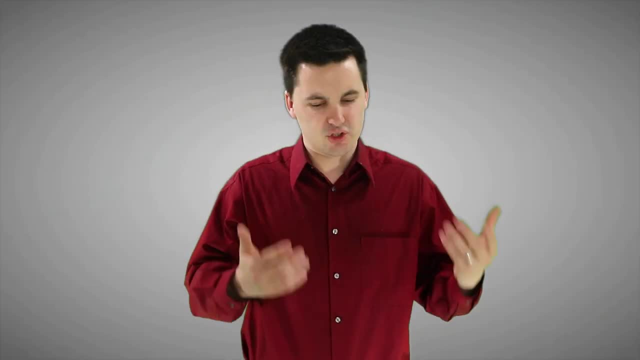 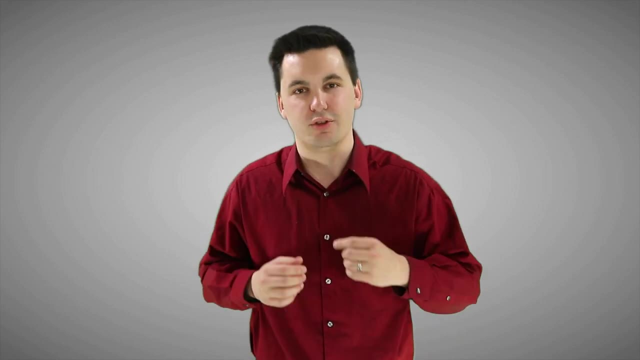 also might influence even foreign policy for certain states. If a state wants to make sure that they can continue to trade with other countries around the world, they'll have to make sure their foreign policy is favorable to their trading partners. Otherwise they might lose that. 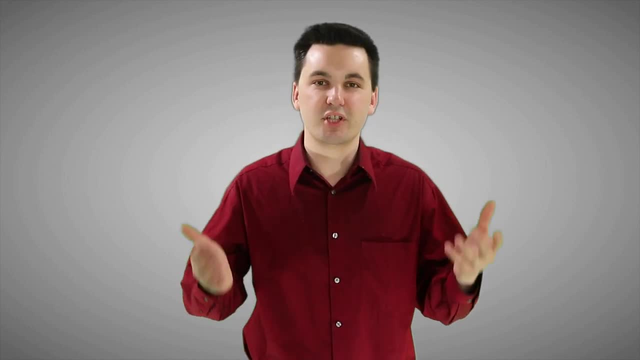 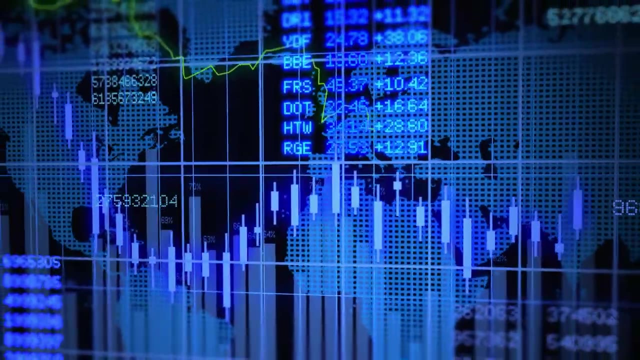 partner and no longer be able to trade with other countries. around the world And on a global scale, we can see just how connected our entire world economy is. It's being influenced every single day by events that occur around the world, And global trade can. 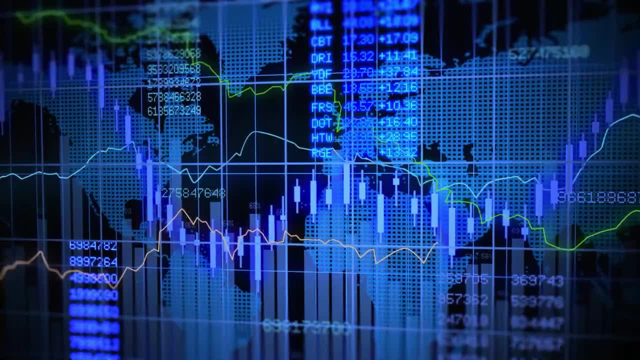 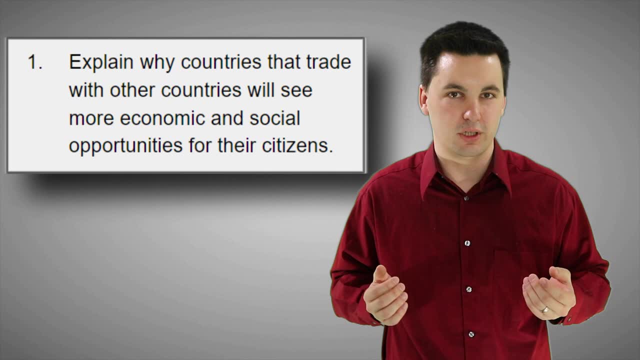 be supported by international trade organizations and, at the same time, hindered by more isolationist policies from different countries. Now we've been talking a lot about global trade and our global community. Take a couple minutes now and review the questions on the screen. Answer the practice. 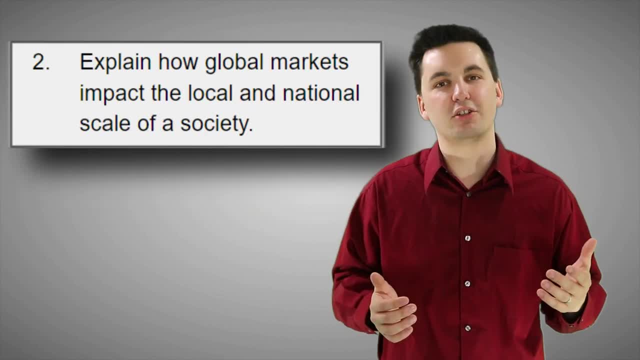 questions and check your answers in the comments below. If you have any questions, feel free to leave them in the comment section below. And while you're down there checking your answers, don't forget to hit that subscribe button. It's free. You can always change your mind later, It's. 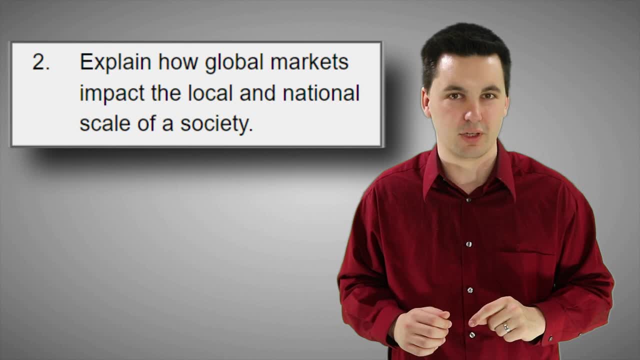 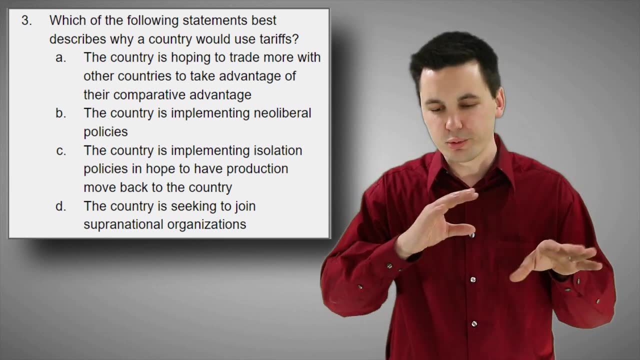 a great way to support the channel and make sure you don't miss out on future topic review videos. And if you do need a little bit more help in AP Human Geography, consider checking out the Mr Synn Discord or my Ultimate Review Packet. Both resources are great. There's a link in the 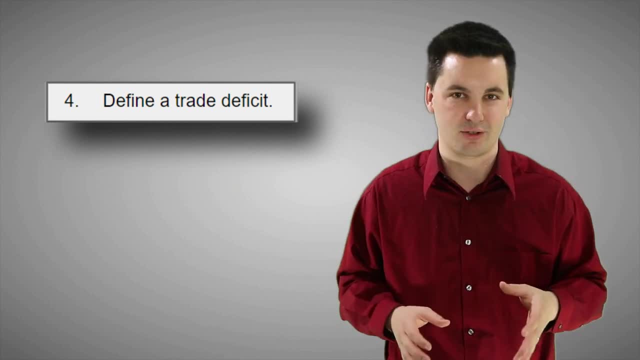 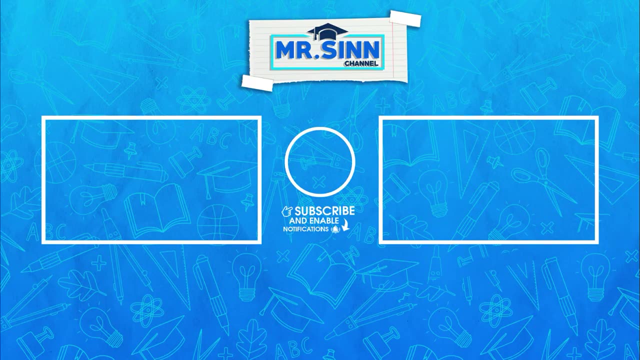 description and it'll help you get an A in your class and also a 5 on that national exam. Thank you so much for watching the Video Geographers. I'm Mr Synn, and until next time I'll see you guys online. Thanks for watching. 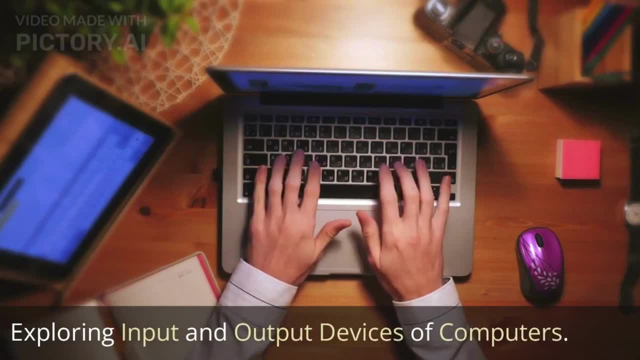 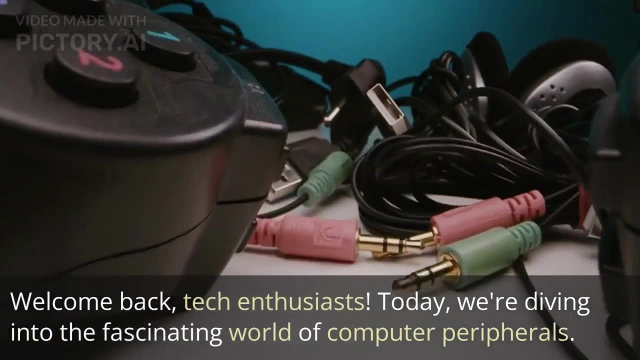 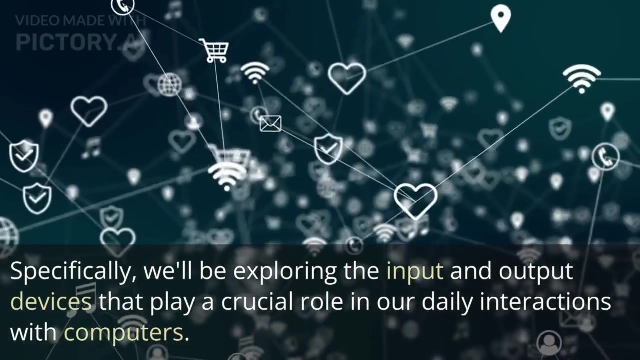 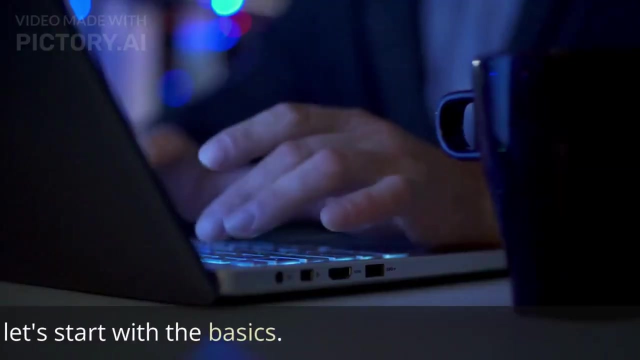 Exploring input and output devices of computers. Welcome back tech enthusiasts. Today we're diving into the fascinating world of computer peripherals. Specifically, we'll be exploring the input and output devices that play a crucial role in our daily interactions with computers. Let's start with the basics.